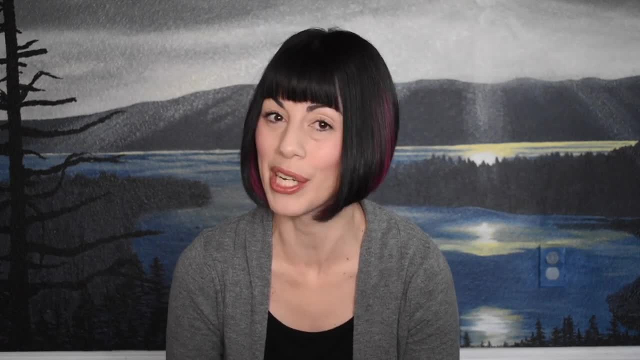 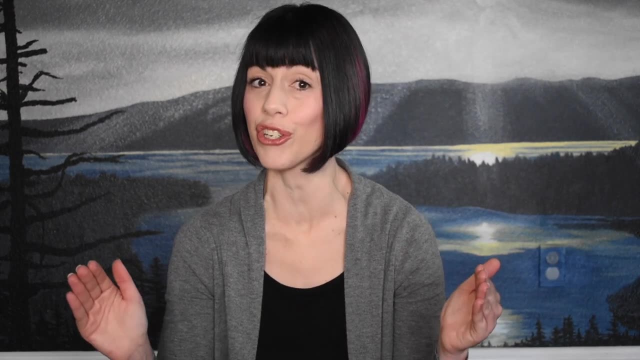 young children or you teach young children. the following errors that I'm going to describe will sound all too familiar. First, it's important to note that if children don't understand that smaller numbers are contained in larger numbers, comparing quantities is going to be much more. 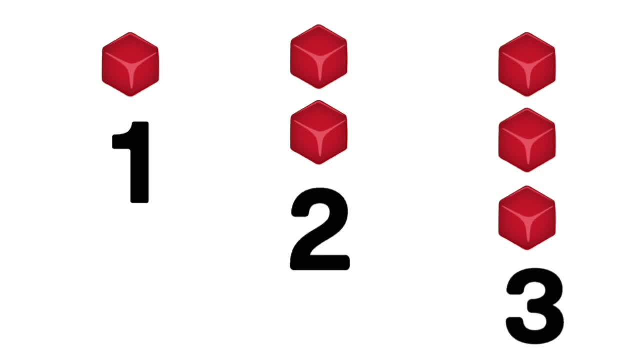 challenging for them. When children first start counting, they believe that all numbers are going to be the same. When they first start counting, they believe that all numbers are going to be the same. When they first start counting, they believe that all numbers are going to be. 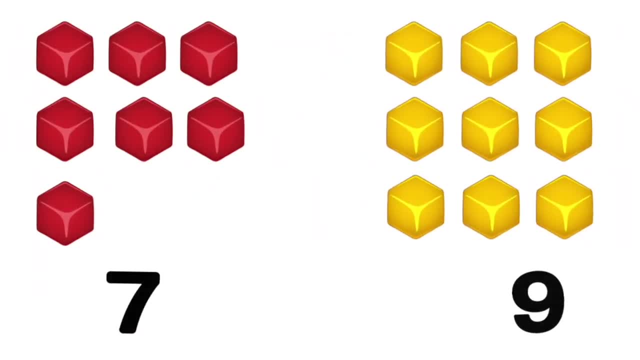 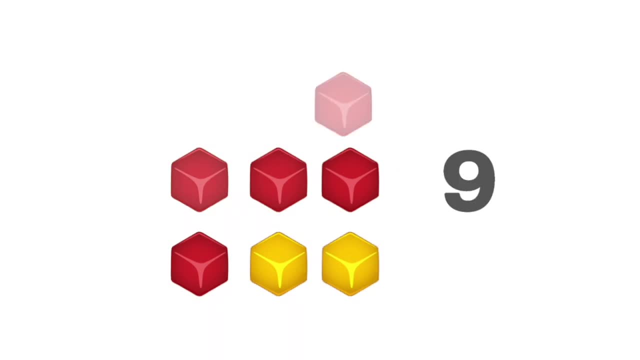 distinct. So seven is seven and nine is nine. They don't yet understand that seven is contained within nine when they count. So how does this relate to the errors that we commonly see when we ask children to compare numbers and quantities? Imagine seeing a set of five blocks in a row. 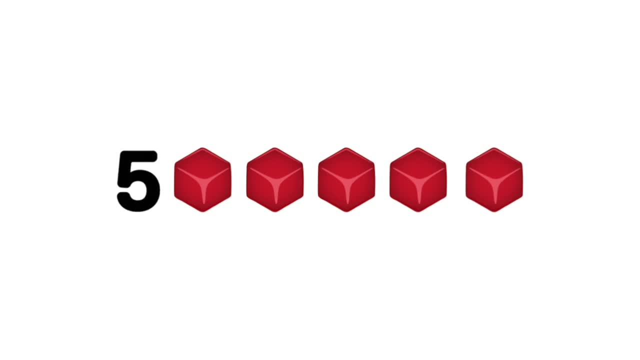 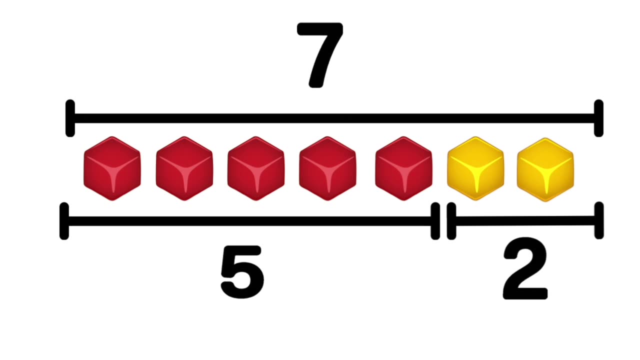 When we ask children to add more, to make a set of seven, one of the most common mistakes they make is creating a brand new quantity rather than adding on to what is already available. This can also happen when you ask a child to change a group of objects to be less. 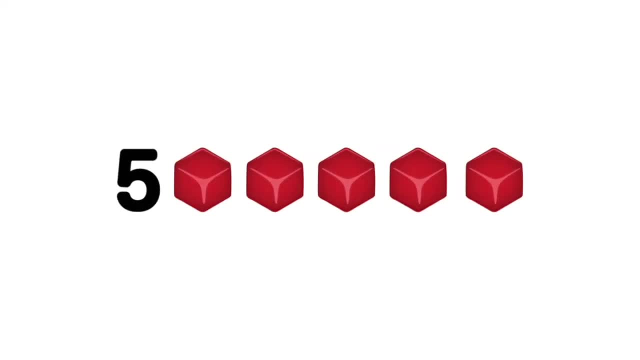 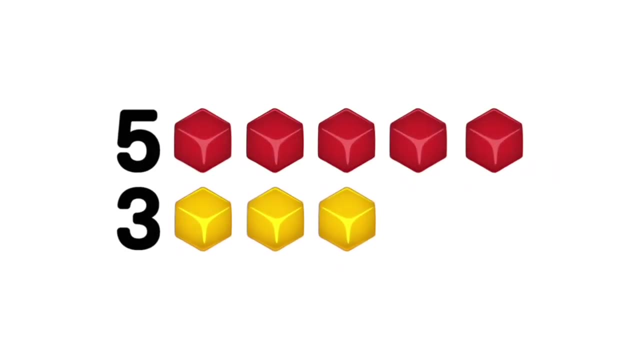 Let's use the same example. Imagine seeing that same set of five blocks. Let's say we ask children to change the quantity to three Rather than removing two. they might build a separate group of three. When we ask them how many blocks they have now, they will likely be. 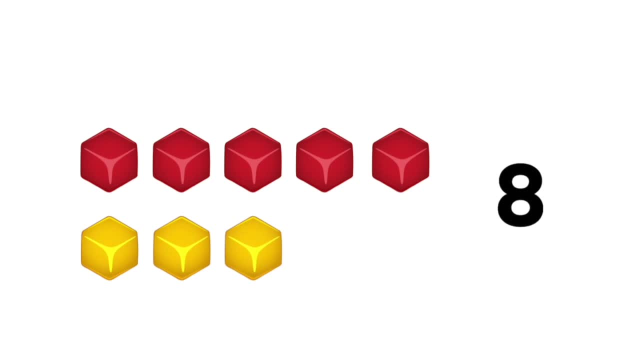 surprised that the answer is eight. I mean, after all, they did exactly what we asked them, right, They made a group of three, but they didn't quite see that all they had to do was remove two in order to get that group of three. In their minds those numbers are still distinct: Five is five and two is nine. 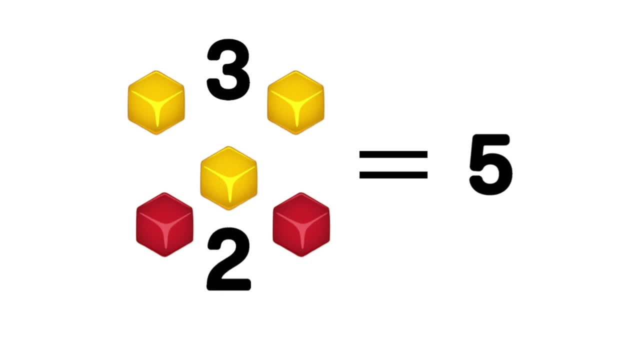 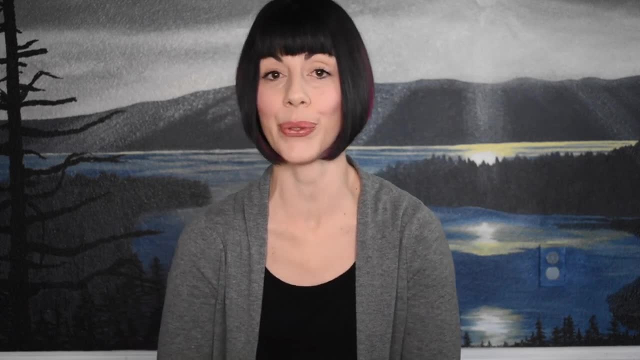 Three is three. They're not yet connected, at least in their minds. This error becomes even more apparent when we move on to more complex questions such as: how many more do you have in this set? Even when children are able to successfully make a change to a quantity. 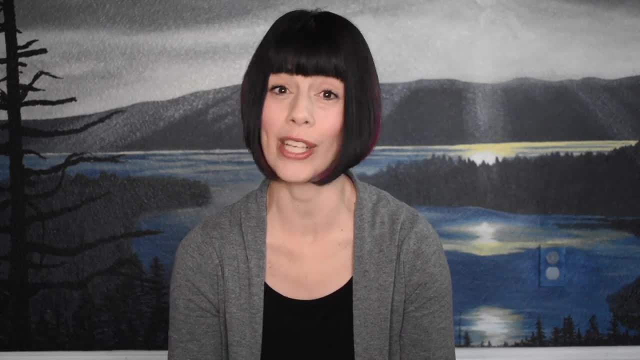 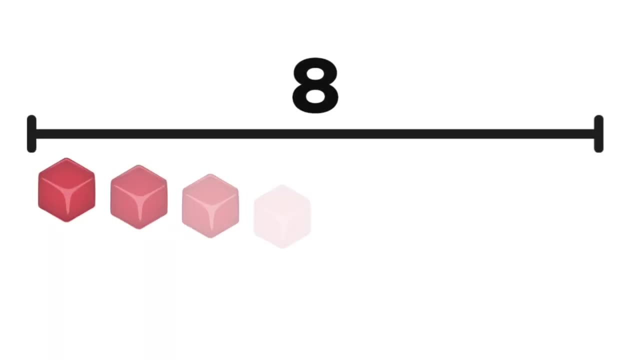 to match what we ask them to do. they still might answer this question incorrectly. If we use the five blocks in a row and ask children to change it to a group of eight, they might be able to add three more. But when asked, how many more does the set have now? they will likely say: 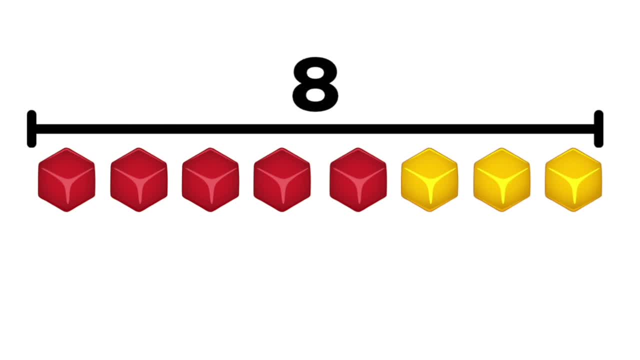 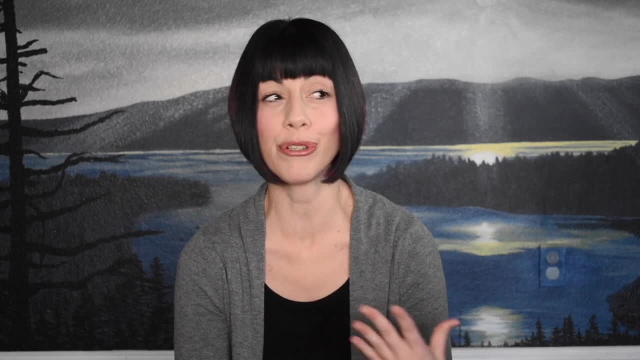 eight more, because eight is the number where they knew they needed to stop. As an educator, this resonates with me so much. Whenever we use the word more to describe quantities, children are generally confused, and for very good reason. More usually means the bigger group, but 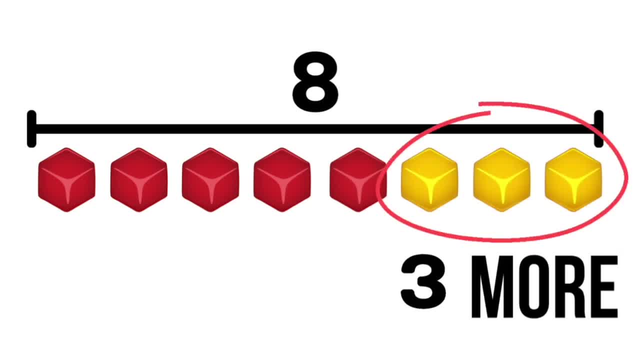 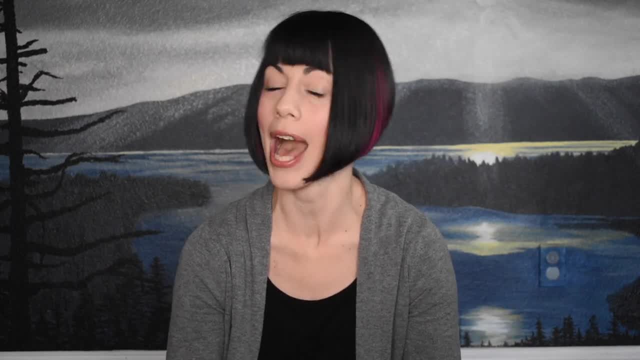 in this sense, we are actually looking for the smaller group of objects. The vocabulary used makes this question incredibly difficult to understand. Try this with your child the next time. you need to know how many more they have in a set Instead of saying how many more. 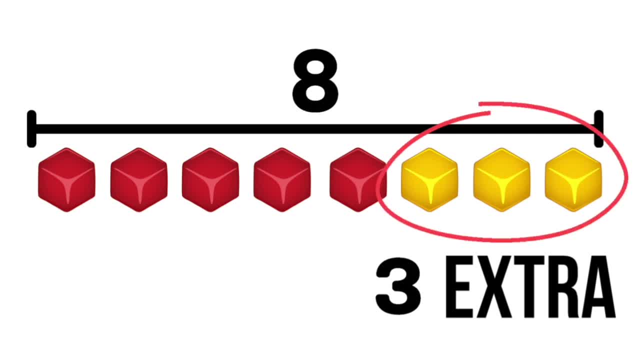 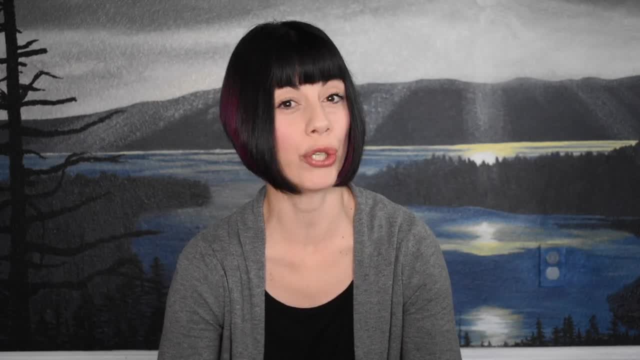 try saying how many extra objects are in this set. Using the word extra instead of the word more makes it more obvious what it is you're asking them to do. So what can we do to support our children if they are struggling to understand the concept that smaller numbers are contained? 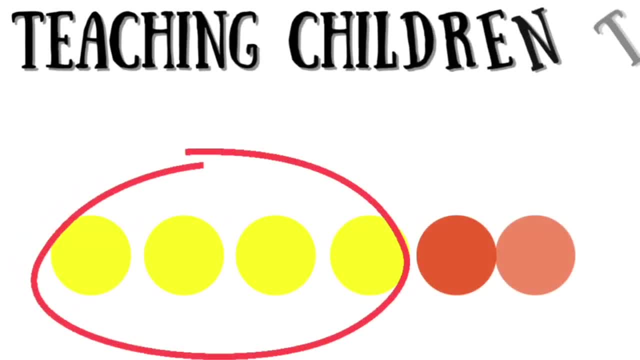 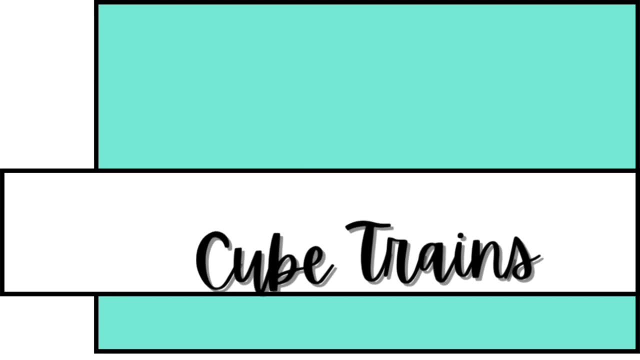 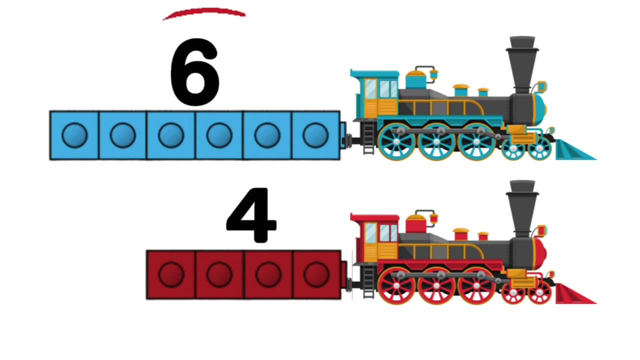 within larger numbers. Luckily, there's a lot of very easy activities you can do to support them in this area. For this activity you'll need some linker cubes. Line up two different amounts of cubes, Have your child count how many cubes are in each train, Then ask which train has more. and 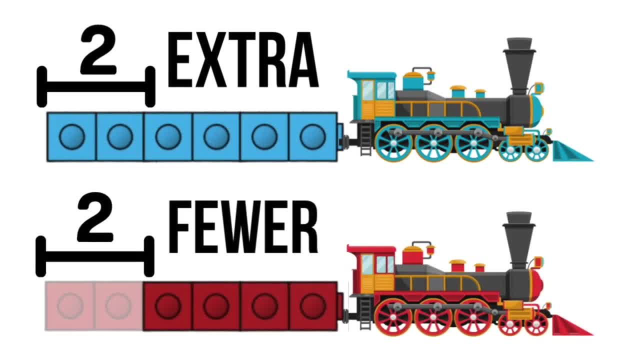 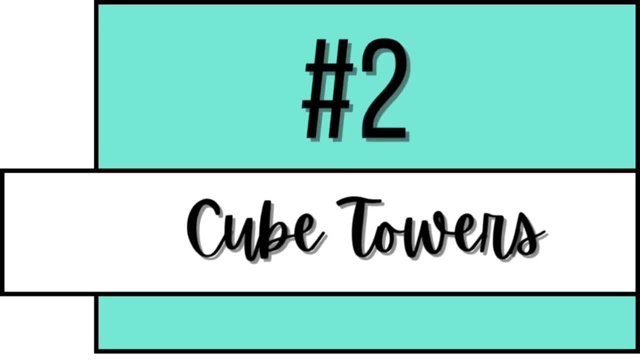 which train has less. Ask how many extra cubes the longer train has, Do this with different quantities and make sure you change up the questions as you build. For this next one you'll need dice and linker cubes. Roll the dice and build a tower to match the number of dots on the dice. 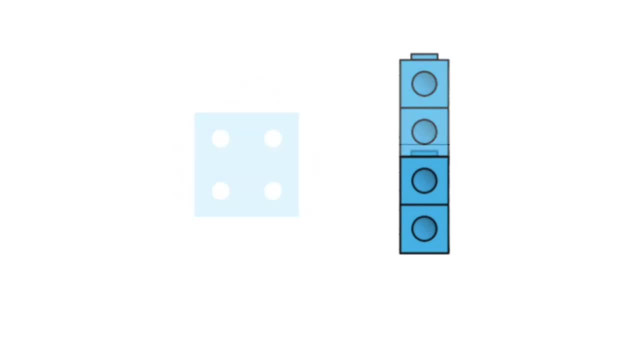 Roll again and build a second tower right next to the first. You can ask your child the same questions you did in the cube train game to give them practice with comparing numbers in order to solve the problem. You can also ask your child the same questions you did in the cube train game to give them practice with comparing numbers in each train. 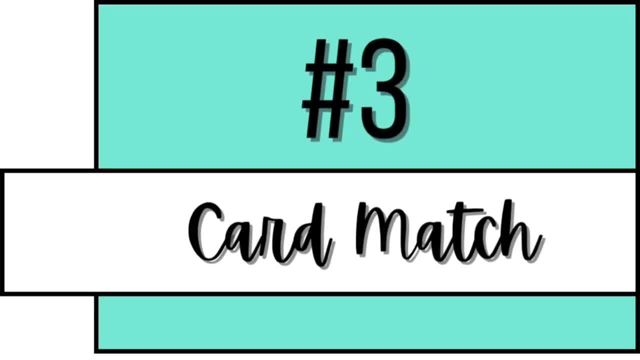 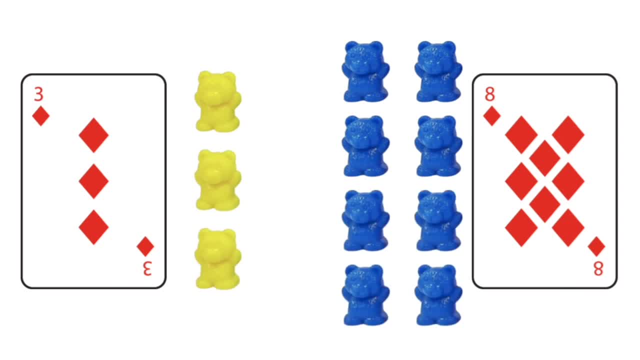 quantities. For this activity you're going to need a deck of cards and a small collection of objects. You and your child will each draw a card. Then you will each build the quantity identified on the card. Make sure you take out the jack, the king, the queen and the ace. Ask your child which group. 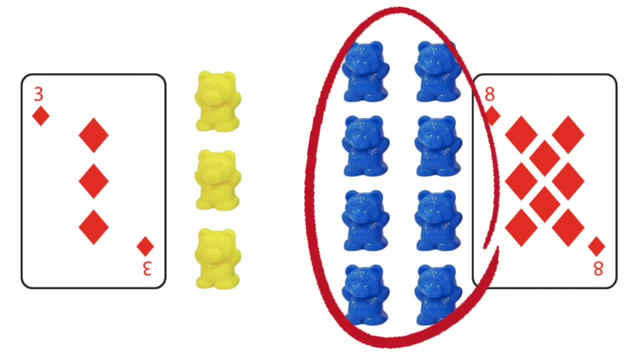 has more and which has less. Whoever turned over the card with more will get to keep both cards. Whoever has the most cards collected at the end of the game is the winner. You can also change the rules and have the person with the least amount on their card be the winner.